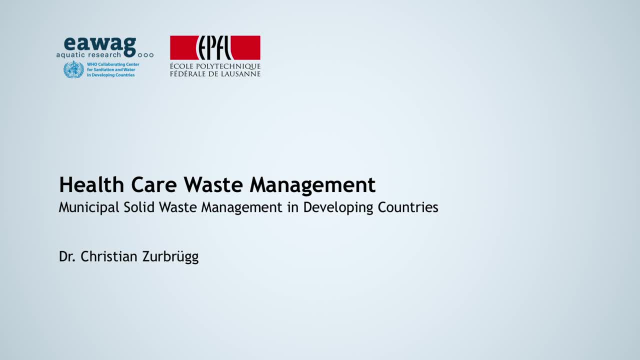 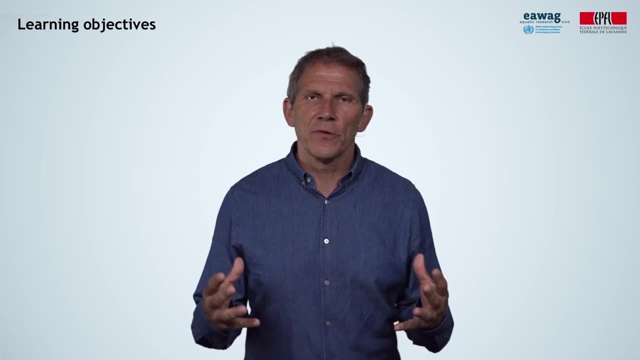 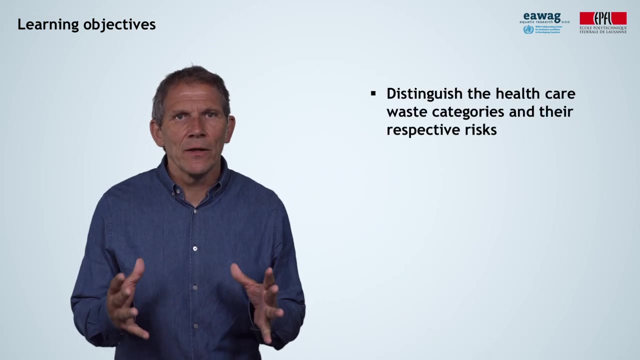 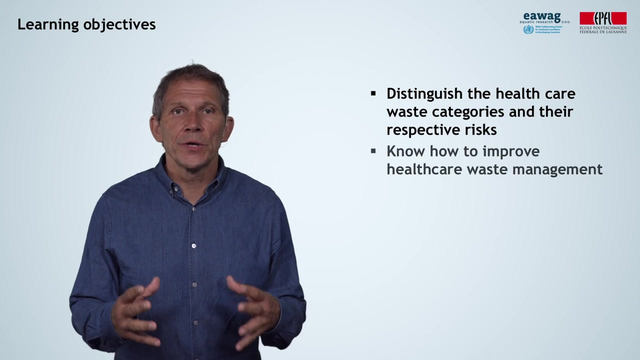 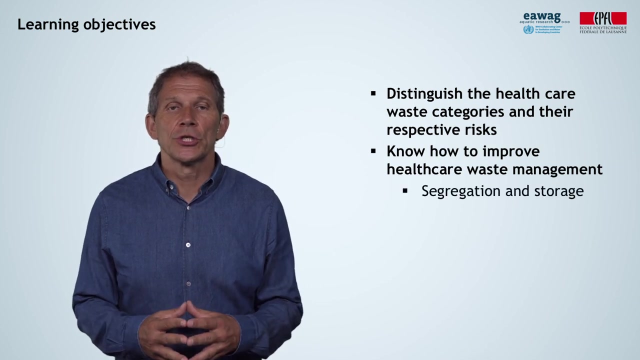 Welcome back. In this module, we'll be covering the very important aspect of healthcare waste management. Hopefully, after this module, you'll be able to distinguish the healthcare waste categories and their respective risks. You should also know how to improve healthcare waste management, especially regarding segregation, storage and treatment. This module is quite 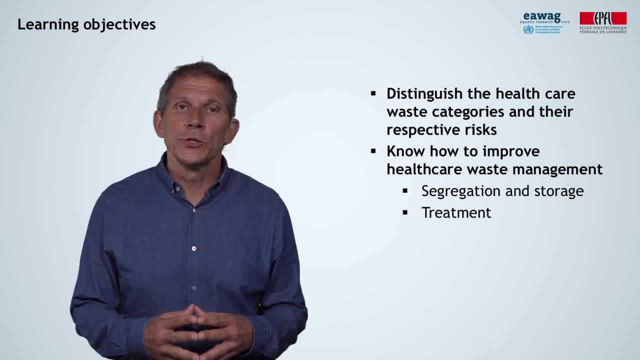 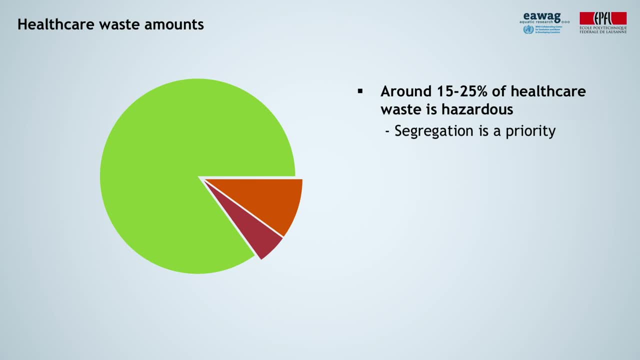 short, so we'll also give indication where you can obtain more information and further training. First and above all, you have to realize that healthcare waste comes from many sources, including major sources such as hospitals, clinics and laboratories, but also healthcare waste management. This module is quite short, so we'll also give indication. 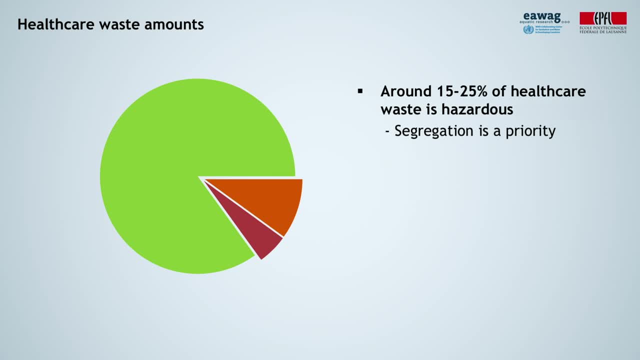 where you can obtain more information and further training. This module is quite short, so we'll also minor sources such as doctor offices, dental clinics and convalescent homes. If we look at healthcare waste amounts and composition, what is most important to know is that only. 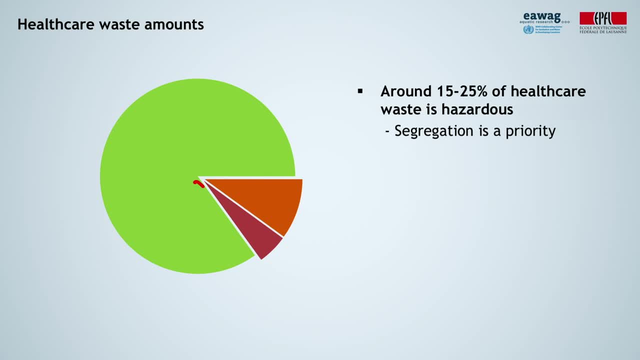 15 to 25 percent of the healthcare waste. only this fraction is actually hazardous. The rest is actually like municipal solid waste and can be treated as normal municipal solid waste is treated. So what is most important is to segregate this hazardous fraction from the rest, because it is this part that needs special treatment. 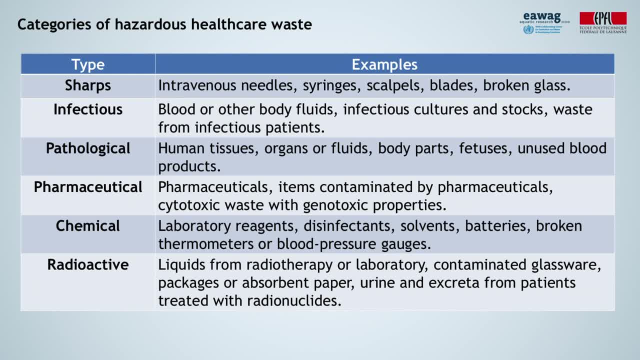 Here is a list of categories of hazardous health care waste, For instance sharps, That's needles and syringes, but also blades. Then there is infectious waste, Blood, body fluids or infectious cultures. Pathological waste, which includes human tissue, organs or body parts. Pharmaceutical waste, which 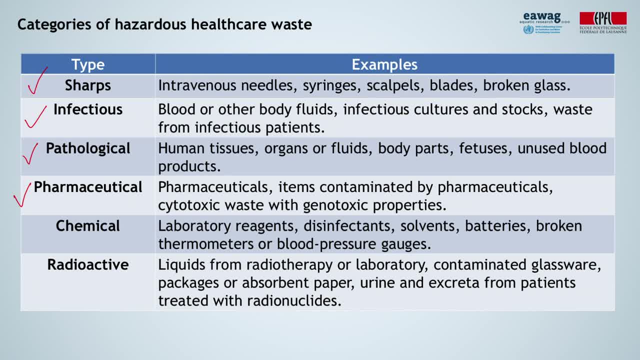 obviously are pharmaceuticals. Then there is chemical waste: Reagents, disinfectants, solvents, but also batteries or thermometers containing mercury, And finally radioactive waste from radiotherapy or pharmaceuticals. Implementing a comprehensive segregation system involves knowing how to distinguish these various fractions and then setting up a system. 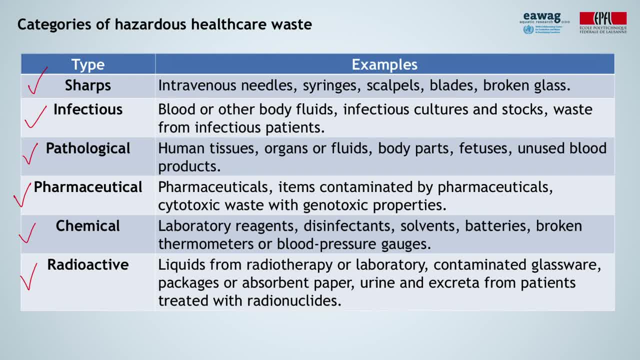 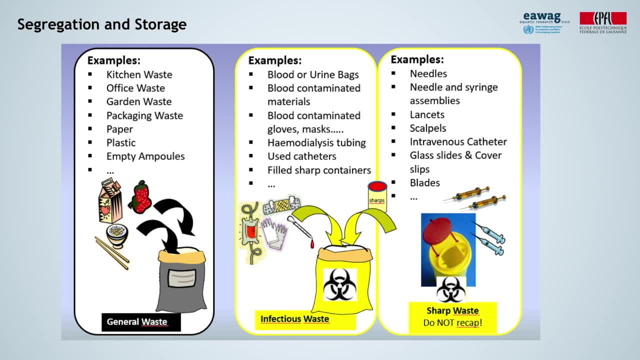 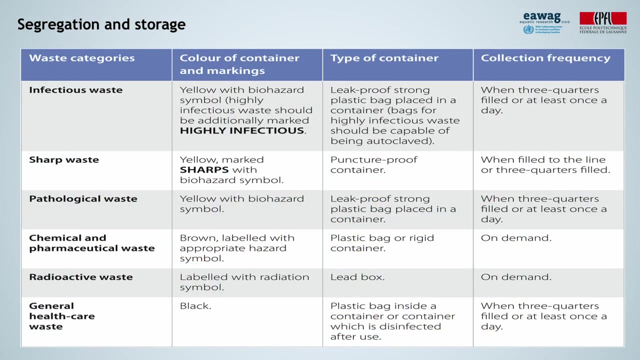 to be able to store these separately. Here is one example of color coding on bins and containers for these different health care waste categories. You see the infectious and the sharps typically color-coded with yellow and the normal waste with black. This is also shown in this table by WHO, where recommendations for color coding and 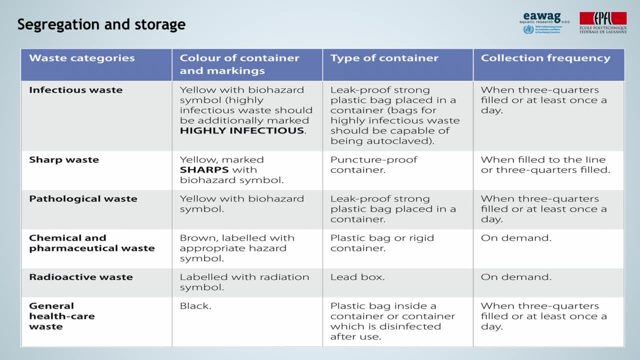 types of containers for the different categories are given. Let us take one look at a specific case of sharps. Sharps is one fraction with a high risk of risk, mostly for health care workers, waste workers or sometimes even users of recycled injection equipment. Here are some examples of sharps containers. They must be. 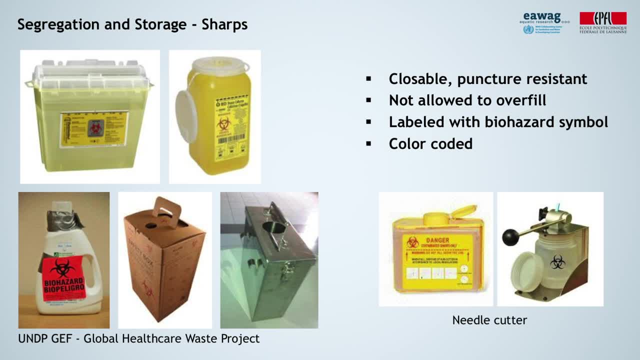 closable, puncture resistant and leak-proof on the sides and on the bottom. They should be accessible, always maintained upright and not allowed to overfill. Also, they should be labeled or color-coded labeled, even with a biohazardous symbol. 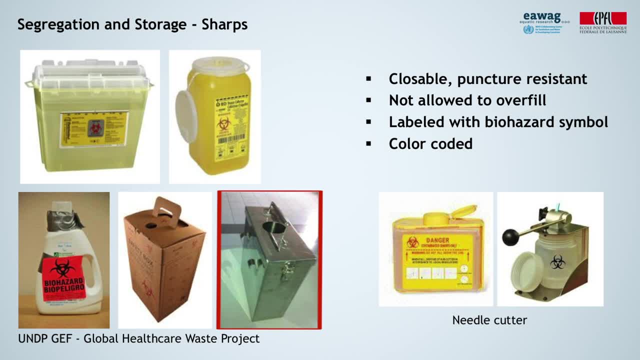 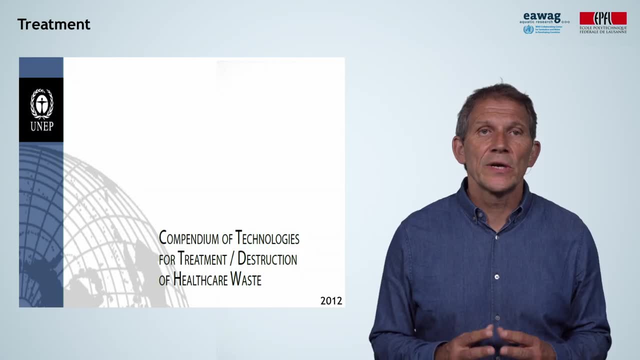 In one example, you even see a container that is suitable for direct treatment in, for instance, an autoclave. Now let's look at health care waste treatment. Health care waste treatment systems are commercially available today. The choice of technology depends on the characteristics of the waste. 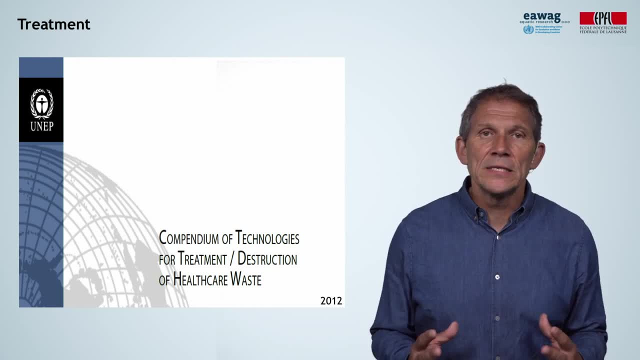 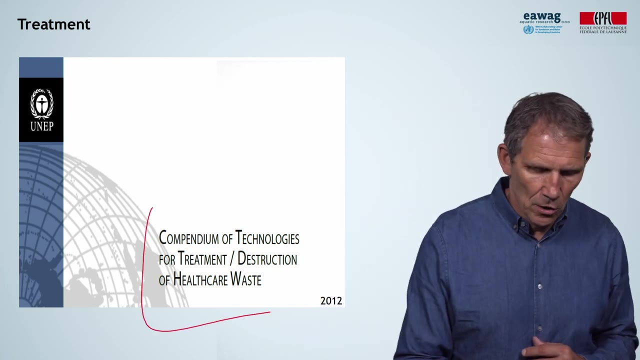 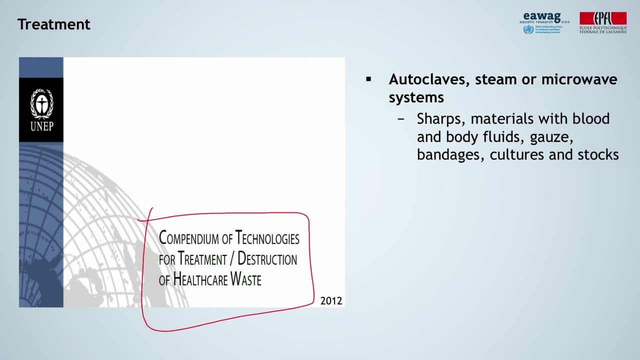 of the health care facility, the capabilities and the requirements of the technology, environment and safety factors, as well as cost. A good overview is given in this document from UNEP on technologies for treatment and destruction of health care waste: The most common types of treatment. 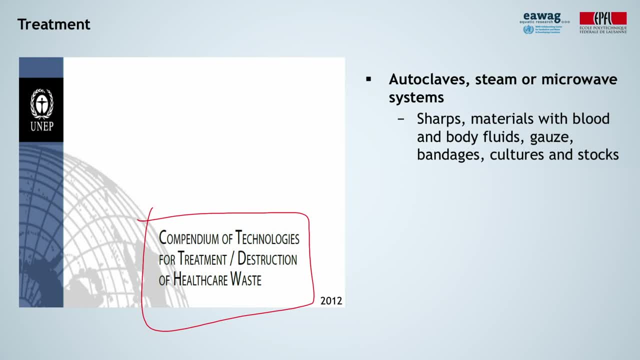 technologies are autoclaves, hybrid systems, steam-based treatment systems or microwave treatment technologies. Then there is also dry heat treatment technologies, where waste is heated up by conduction or thermal radiation. This requires higher temperature and longer exposure times than steam-based processes. They are commonly used to treat small volumes. Then, finally, there is, of course, 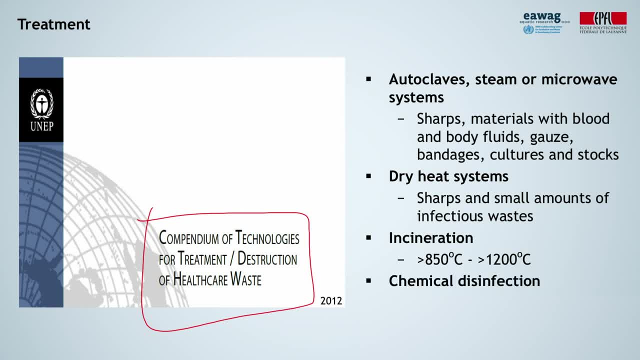 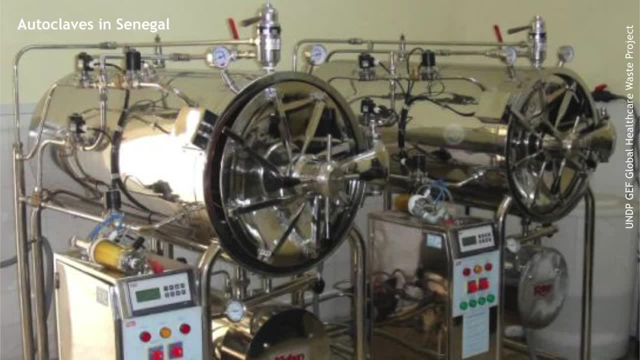 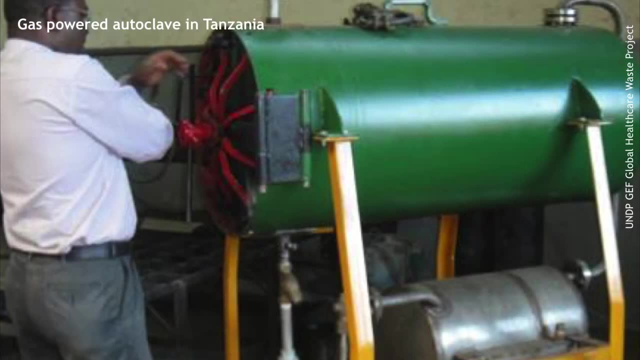 also incineration. There is chemical treatment or options for special landfilling and disposal. Here is an example of an autoclave system in Senegal. Or here another example from Tanzania. In this case this shows a gas-powered autoclave. Then there is also incineration, One simple. 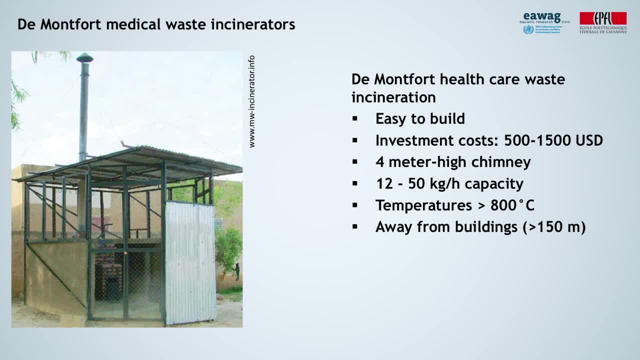 incineration system is the de-molding. This is a manfor incinerator. as a cheap but effective incinerator which can be built in almost any developing countries. It reaches the criteria of a temperature above 800 degrees with a residence time. 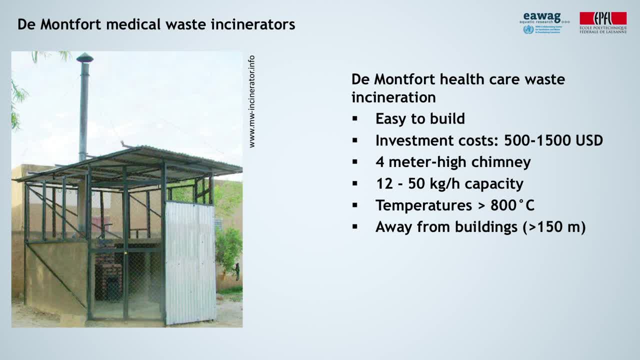 of over one second. Despite that, they've been designed to be simple and affordable, we still have to think of appropriate location and using the right right materials for construction. Guidelines on how to construct, use and maintain such an incineration unit can be found online. The incinerator should be built at a convenient distance away from buildings so that any smoke or gas does not enter the buildings. 150 meters is the suggested minimum. So now, how do we go about to set up a system, for instance at a hospital? First of all, we need to take into account the legislative framework. 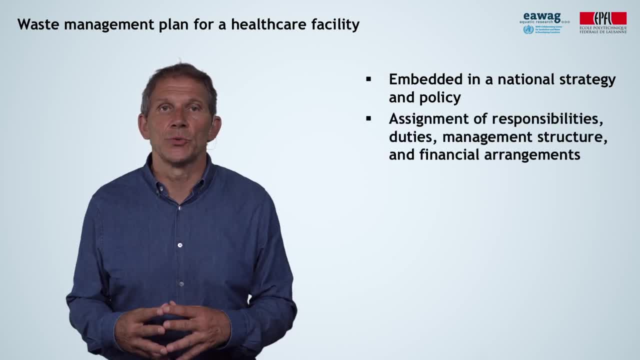 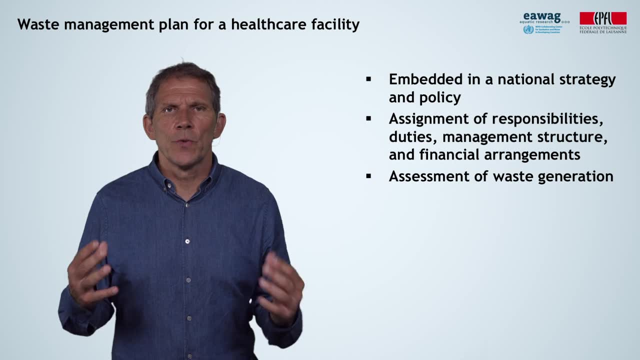 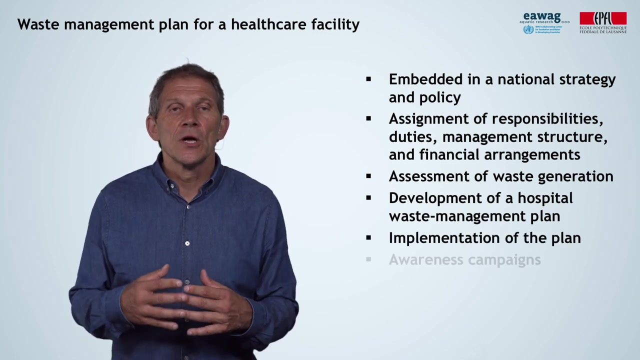 We also need to assign responsibilities and duties, find financial arrangements, But also we need to start by knowing our situation through monitoring and an assessment, And based on that, we can then develop a waste management plan and implement this through appropriate infrastructure and, of course, with an intense development of awareness through. 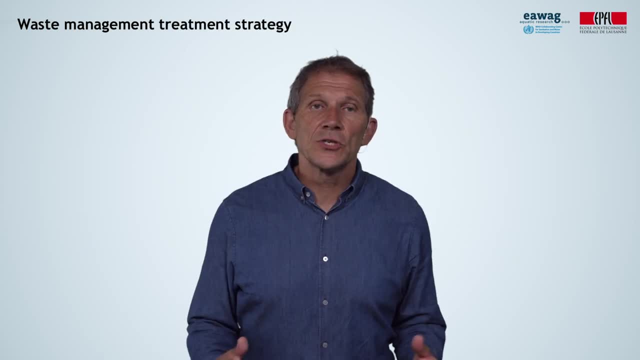 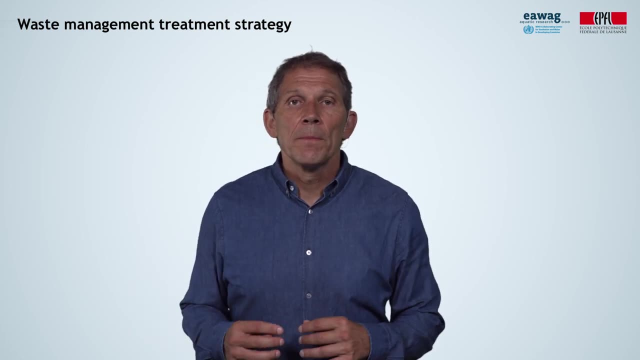 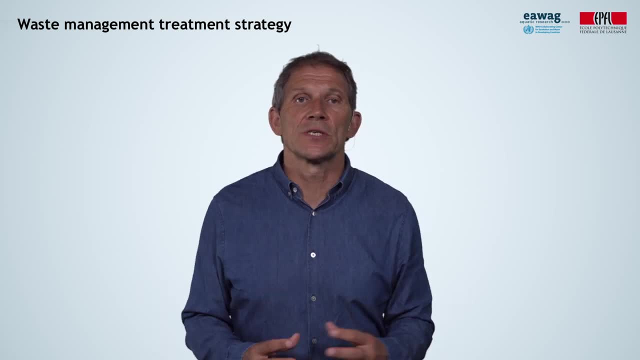 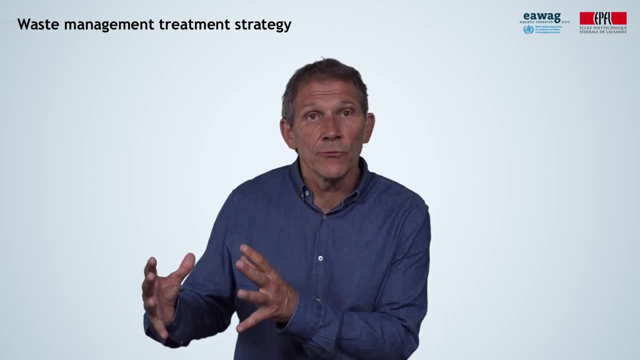 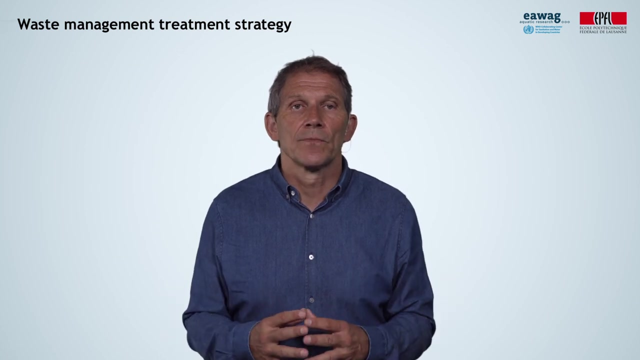 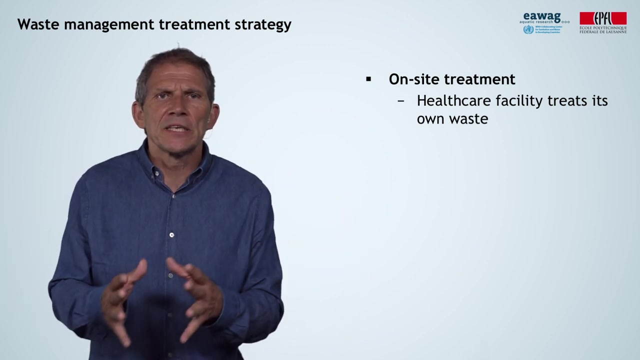 able to manage healthcare wastes from different sources. The aspects of segregation will happen at the healthcare center itself, but then how to organize transport and treatment might take different pathways. For instance, if the healthcare facility is large, like a central hospital, then treatment can happen at this same location. On the other hand, for small center, 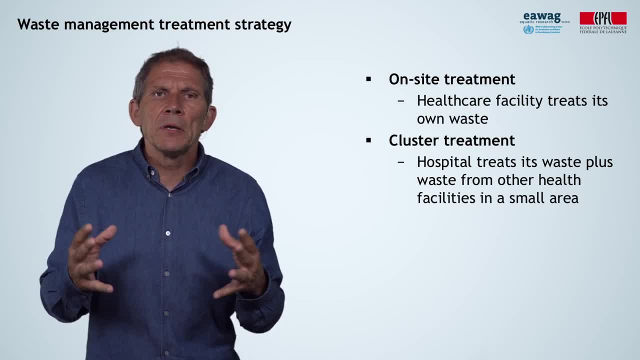 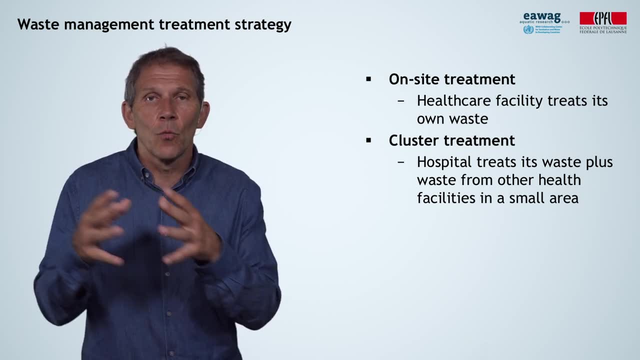 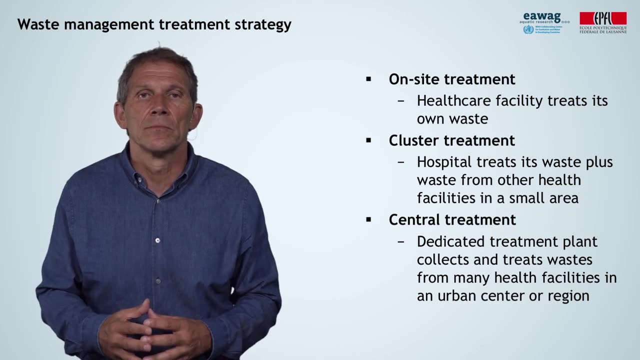 which are distributed all throughout the city. it will probably make more sense to set up a collection and transport system and then have a semi-central treatment at one larger facility or even a central treatment at one specific location in the city. So to summarize, in this module we have looked at 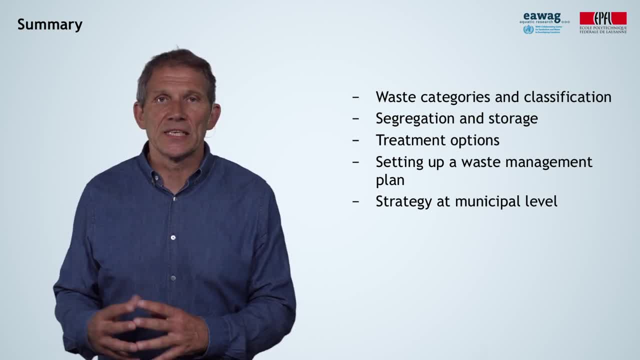 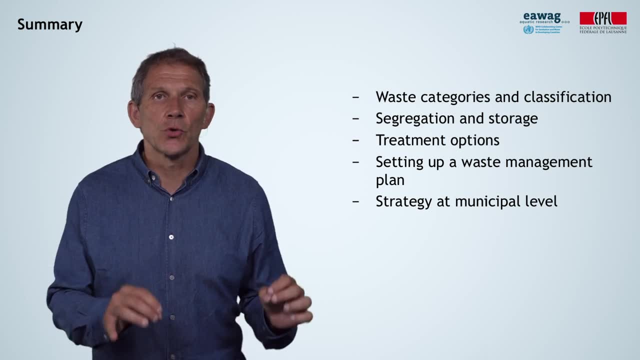 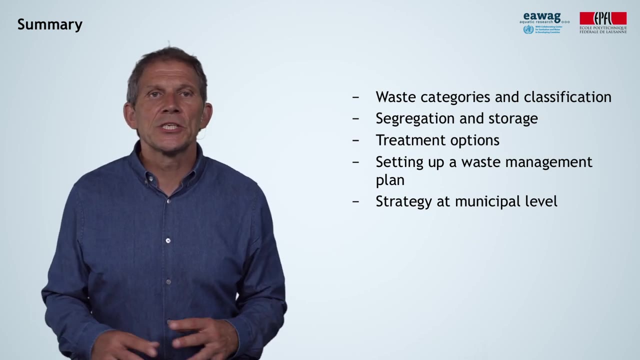 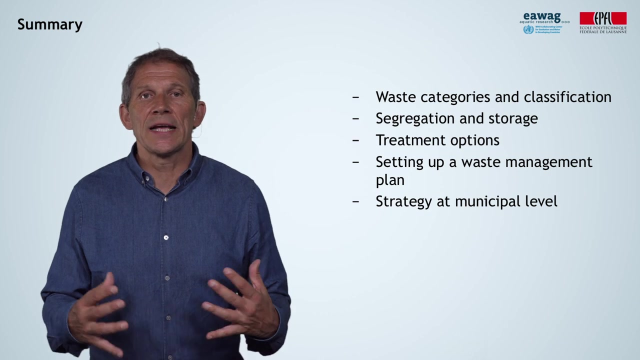 healthcare waste, its different categories and risks. We have discussed aspects of segregation at source, specifically also the site storage requirements. Then we looked at some examples of treatment options and then concluded by describing some elements of planning for healthcare waste management at the facility itself, but also taking an overall perspective on how to plan for a citywide solution. 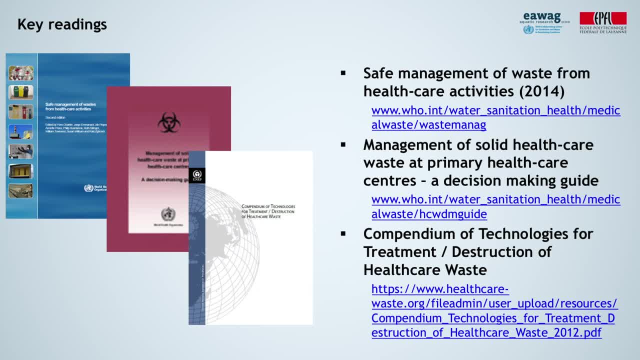 If I have been able to excite you about healthcare waste management and you feel now disappointed that this module just gave you a small glimpse of the issues, then I can recommend the following documents for further reading. As you can see from the website links, it is WHO, the World Health Organization. 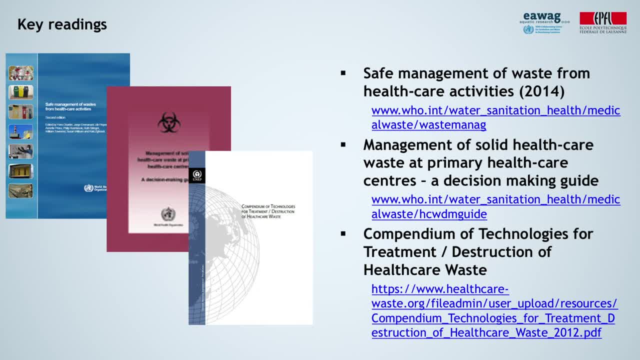 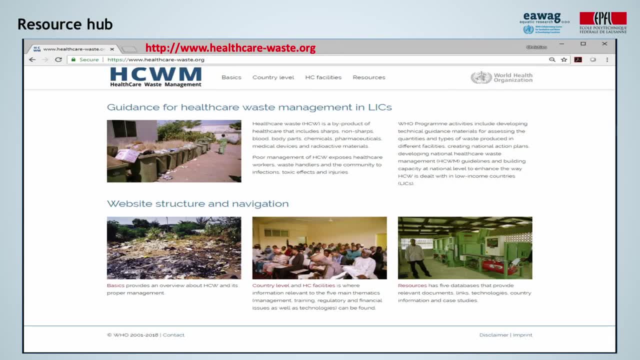 that has quite a number of very exciting documents that make for an interesting read. Also, this web page by WHO is a resource hub for very many different issues related to healthcare waste management. We have links to basics, there are aspects of country issues and